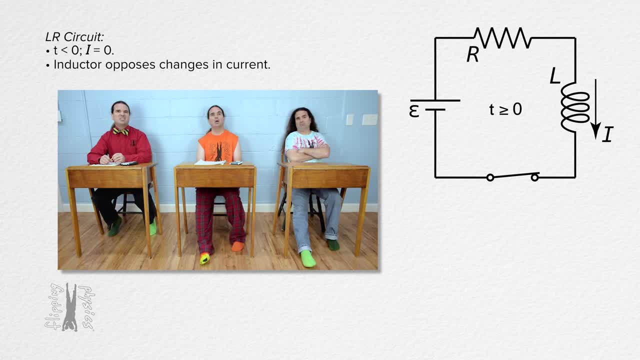 oppose changes in current. We talked about that last time. Yeah, The inductor opposes changes in current in the circuit. So because there was no current in the circuit before the switch is closed, right when the switch is closed, the current is initially. 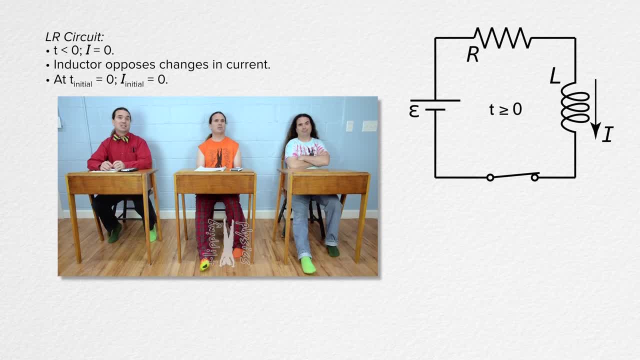 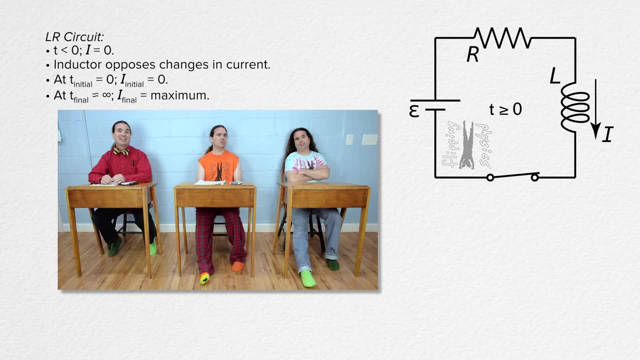 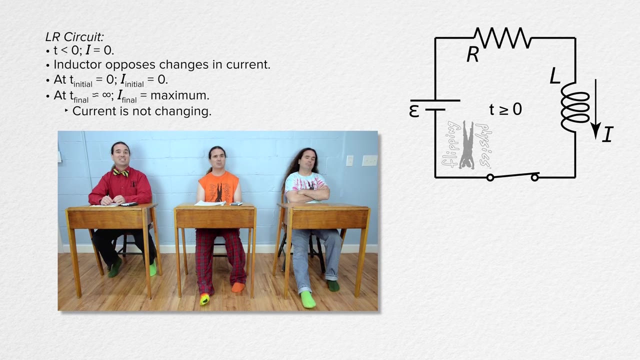 zero. But After a long time the current will have increased to its maximum current and will stay at that current, The steady state current Right. So after a long time the current in the circuit is not changing. so the inductor has no change in current to oppose. So it's basically like the inductor. 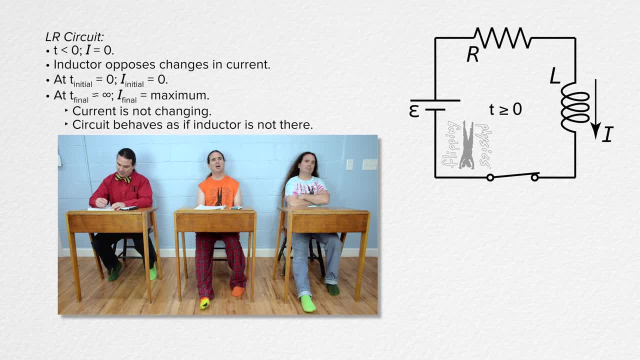 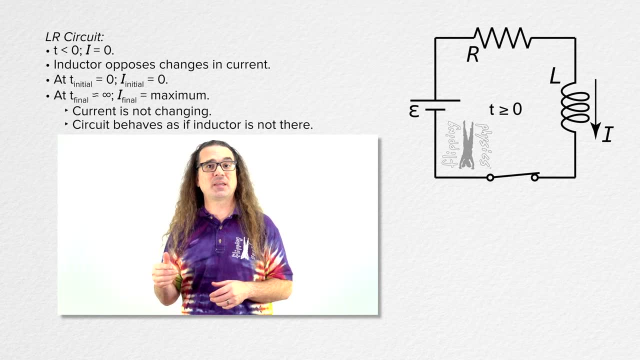 is not there after a long time. Correct: The current at time equals zero is zero And the current after a long time is at its maximum value because the current in the circuit is no longer changing. It has increased to a steady state current and the inductor has. 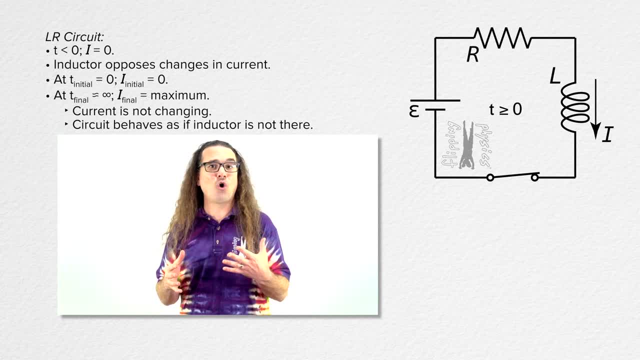 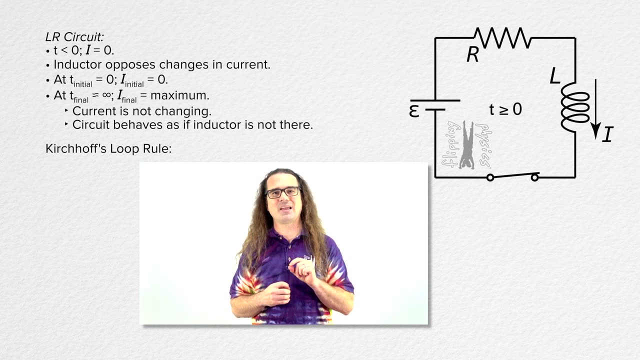 zero resistance to the current, because the inductor is made of a coiled-up ideal wire with zero resistance. But we can actually determine the equations for the limits. To do that, Bobby, please apply Kirchhoff's Loop Rule to the circuit starting in the lower left-hand corner. 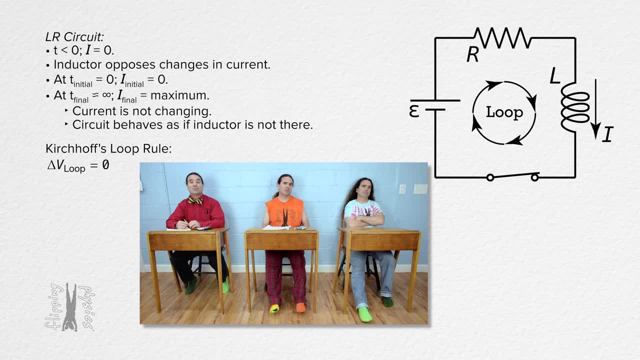 Well, Kirchhoff's Loop Rule states that the electric potential difference around a loop equals zero. Starting in the lower left-hand corner and moving clockwise in the direction of current, that equals. well, we add the emf of the battery because the electric potential difference across 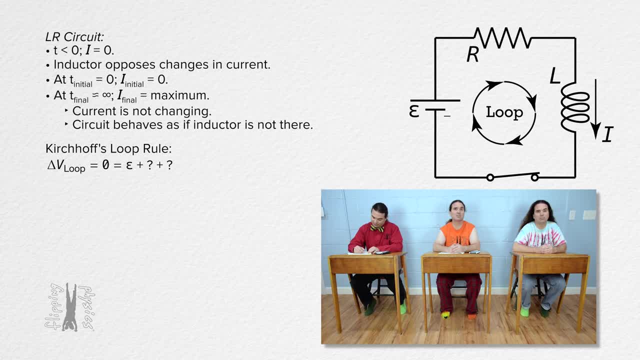 the battery in the direction of the current is from the negative terminal to the positive terminal across the battery. In other words, the electric potential increases across the battery in the direction of current. Then we subtract the electric potential difference across the resistor because the electric potential decreases across the resistor in the direction of the current. 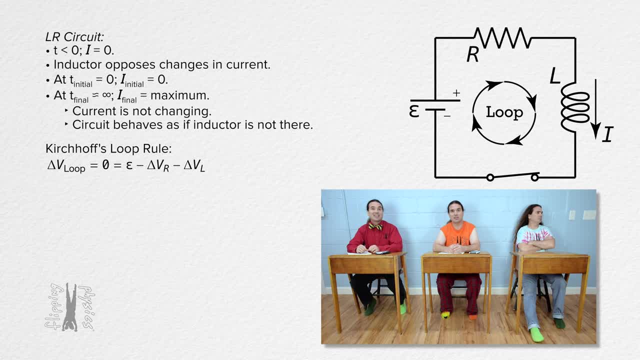 And we subtract the electric potential difference across the inductor because the electric potential also decreases across the inductor in the direction of current when current is increasing, as it is here, And we can substitute current times, resistance in, for the electric potential difference across the resistor and inductance times, the derivative of current with respect to. 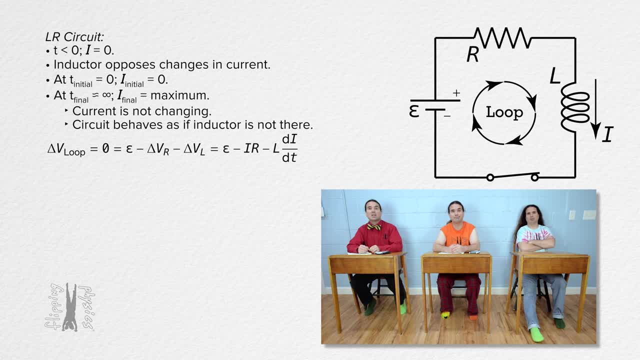 time for the electric potential difference across the inductor. I thought the induced emf across an inductor equaled the negative of inductance times the time rate of change of current. Why did you not include the negative when substituting in the equation for electric potential difference across the inductor? 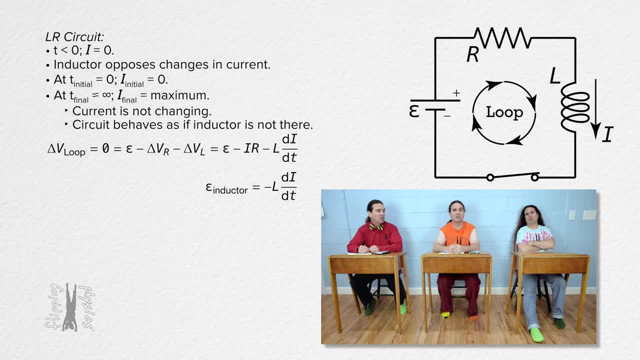 Because we already showed, the electric potential difference across the inductor goes down in the direction of increasing current through an inductor in the Kirchhoff's loop rule equation. If we included the negative from the induced emf equation that would make it so the electric 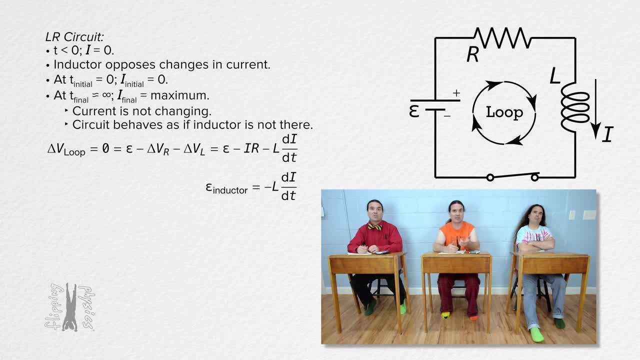 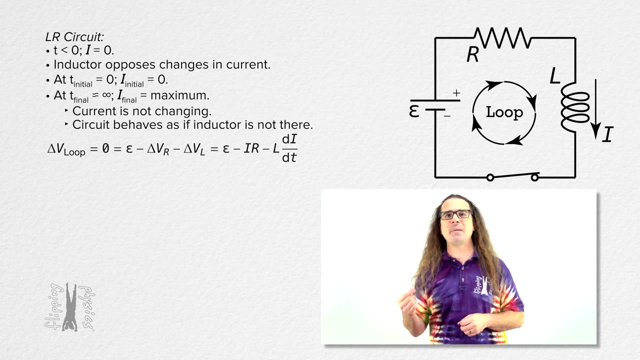 potential across the inductor would go up across an inductor in the direction of current when it is increasing, which does not make sense. Yeah, Well done, Thanks, Billy. please use the equation Bobby just gave us to determine the remaining limits for this LR circuit. Absolutely Well, we know that at the time, initial time, t equals zero. 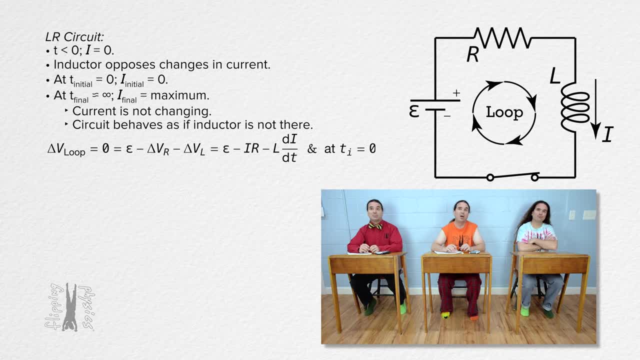 the initial current equals zero. When we substitute that into the Kirchhoff's loop rule equation we get zero equals emf minus inductance times, the derivative of current with respect to time. We can also substitute that into the Kirchhoff's loop rule equation. 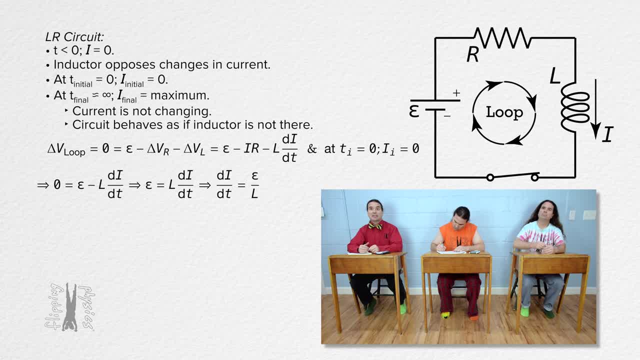 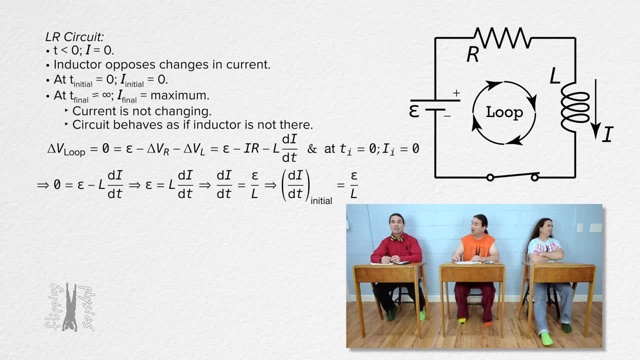 We can rearrange that equation to get that the derivative of current with respect to time equals emf divided by inductance. In other words, the initial value for the time rate of change of current in the inductor equals emf over inductance. 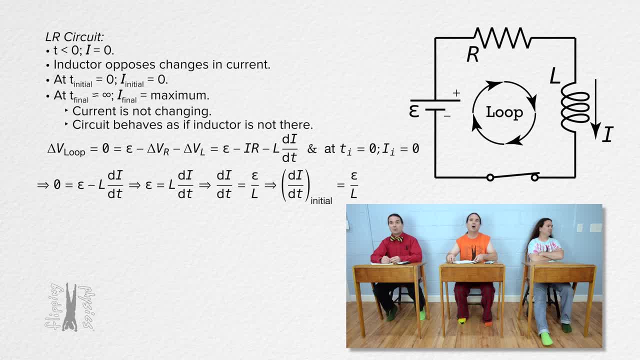 We also know that after a long time or time is roughly equal to infinity- the final time rate of change of current in the circuit equals zero. When we substitute that into the Kirchhoff's loop rule equation we get zero equals emf minus current. 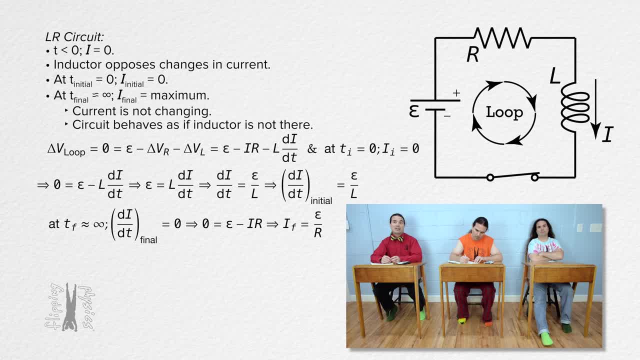 over inductance. We can rearrange that to get current final equals emf divided by resistance. In other words, our limits for current are that it starts at zero and increases to emf divided by resistance, And that means emf divided by resistance is the maximum value. this circuit 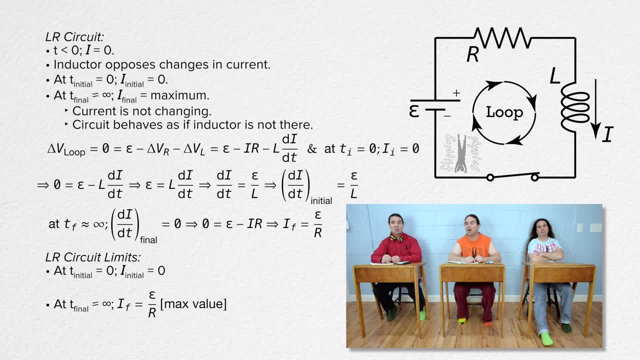 will have. As we said earlier, after a long time the circuit behaves as if the inductor is not there, because this is the value the current in the circuit would have if there were no inductor, And the other limits are that the derivative of current with respect to time starts at a value of 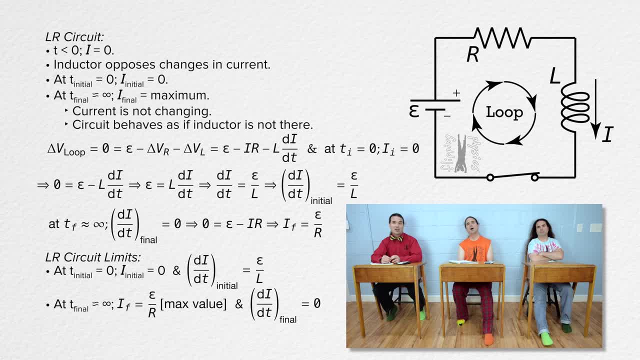 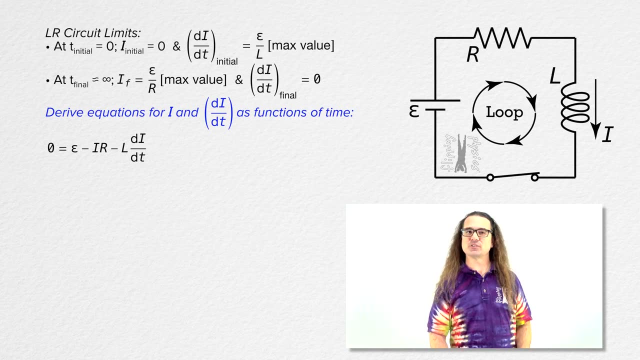 emf divided by inductance and decreases to zero. And that means emf divided by inductance is the maximum value the time rate of change of current will have in this circuit. Thank you, Billy. And now, the moment we have all been waiting for, We are going to derive the equations for 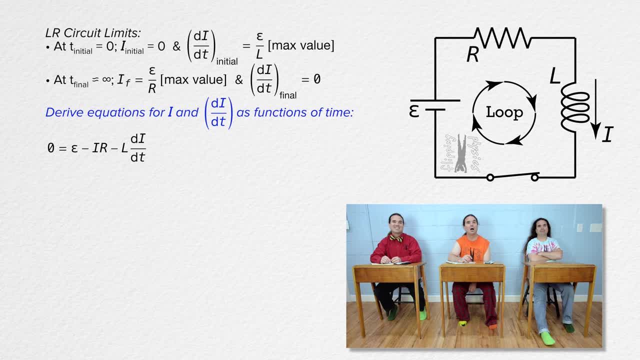 current as a function of time and the time rate of change of current as a function of time. Who's been waiting for that? Uh, I have Me. I've been waiting for that. Then let's get it started in here. 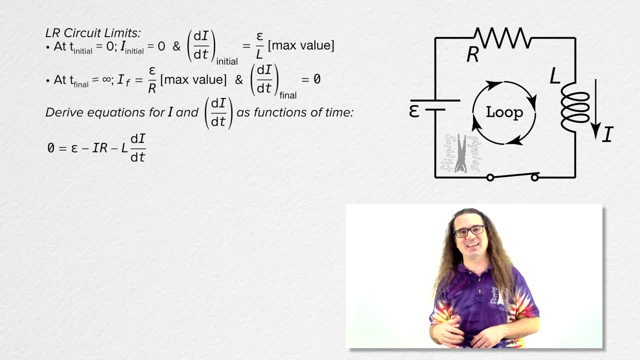 Before we get started, So many preambles, Yeah, well, there's a lot to understand here. You're telling me: Yes, Yes, I am Okay. Before we get started, please realize these derivations are very similar to the derivations. 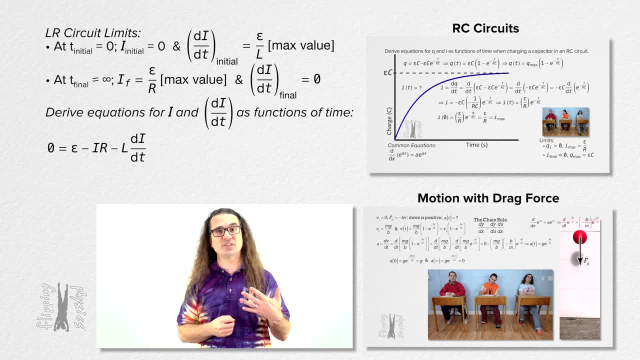 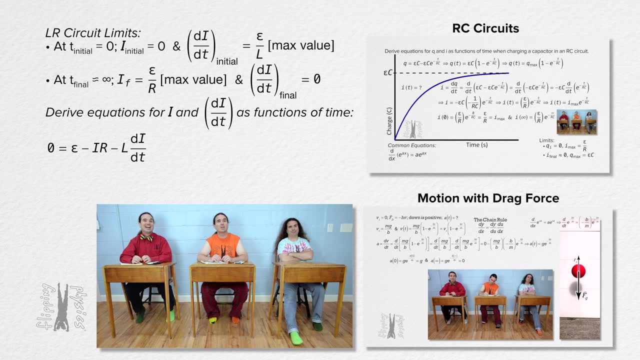 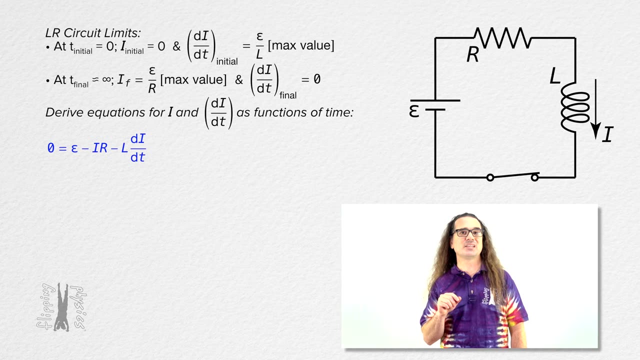 we did for resistor-capacitor circuits or RC circuits, and the motion equations with a drag force. Oh boy Yeah, Here we go, Going back to the Kirchhoff's loop rule equation for this LR circuit, Zero equals emf minus current times, resistance minus inductance times, the time rate of change. 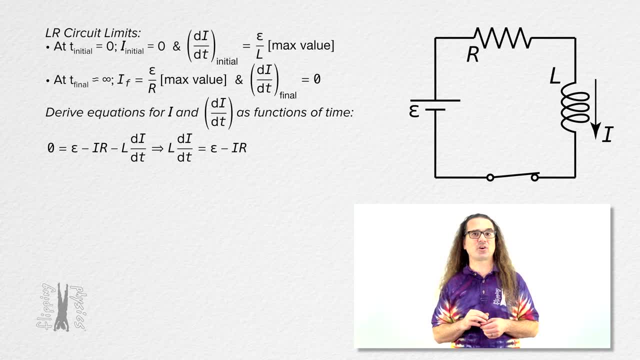 of current. We can move inductance times, the derivative of current with respect to time, to the left-hand side of the equation And we now divide the whole equation by resistance And now we are going to use u-substitution, U-substitution. 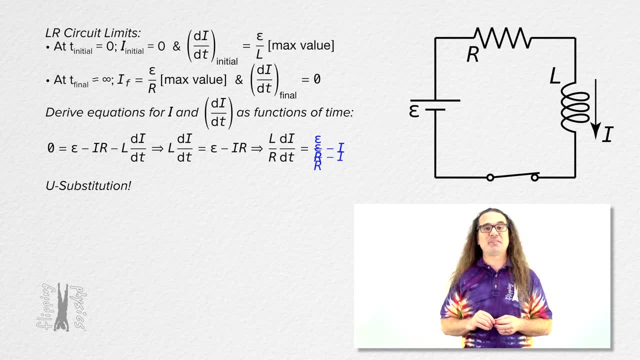 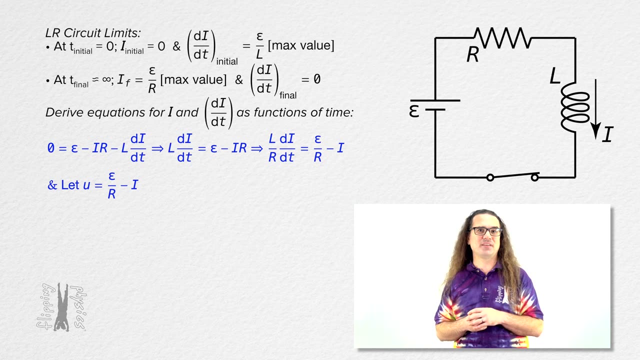 U-substitution. U-substitution: We let the variable u be equal to emf divided by resistance minus current. Now I will say that these initial steps, including the u-substitution, are the ones which are the easiest to forget in this derivation. So I do suggest you. 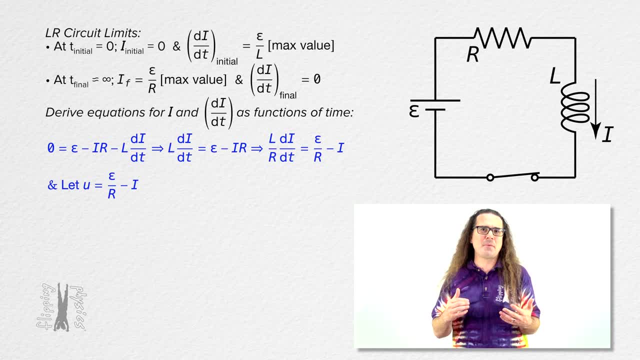 indicate somehow in your lecture notes to specifically remember those initial steps, Please. Well done, Sure Lecture notes. Now Reelize: we have the derivative of current with respect to time in our equations. That means we need to be identifying infinitesimally small changes in variables. 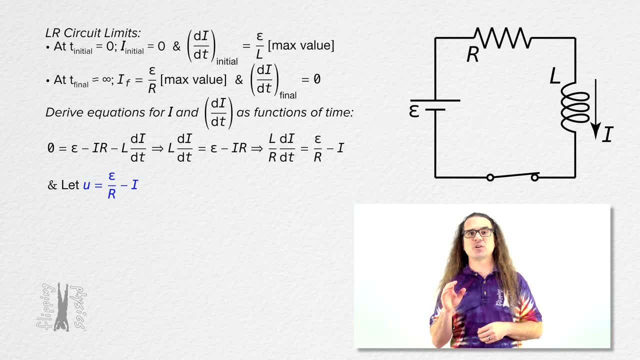 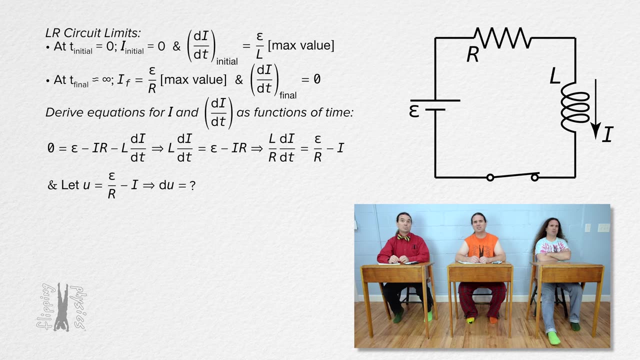 in these equations. Looking at the equation, variable u equals emf divided by resistance minus current, if we identify the infinitesimally small change in variable u or DU, Bobby, what is DU equal to? Uh, DU is equal… to well, emf and resistance are constants, which means they do not change over time. so 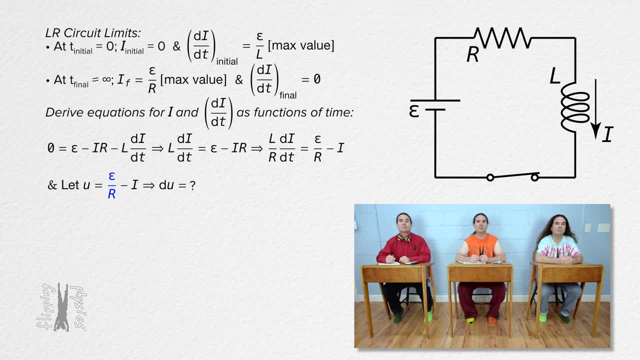 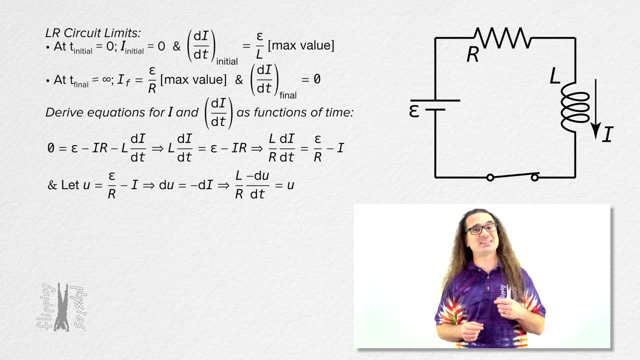 there is no change in emf over resistance. So the infinitesimally small u or du equals the negative of the infinitesimally small current or di Right. Correct, Bobby. And when we substitute u and negative du into our equation, we get inductance divided by resistance. 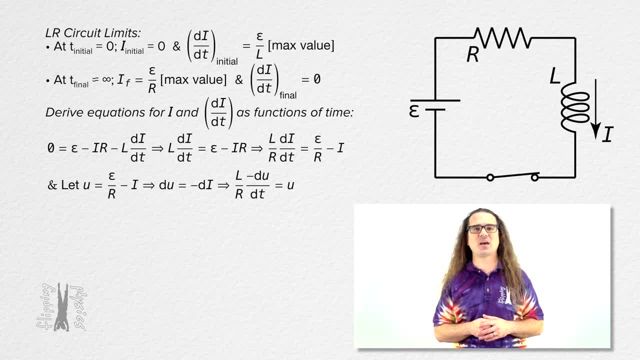 equals the negative of the derivative of u with respect to time. all equals u. And then rearrange the equation to get u and du on the left-hand side and everything else on the right-hand side. We now have du over u equals the negative of. 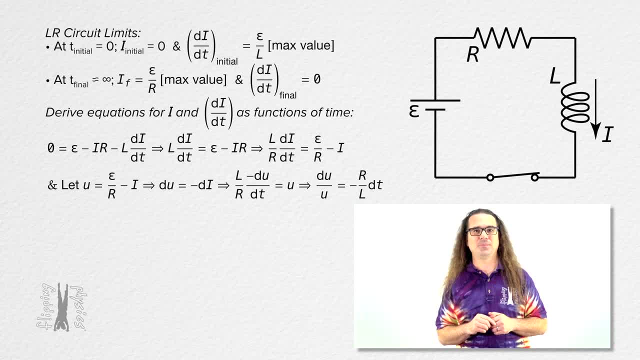 resistance divided by inductance times, dt. And now we can take the integral of both sides And we need to identify the limits on both integrals. The limits on the integral on the left-hand side are the limits on the right-hand side? The limits on the integral on the left-hand? 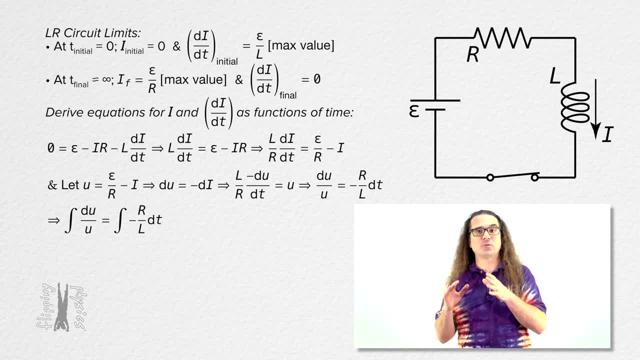 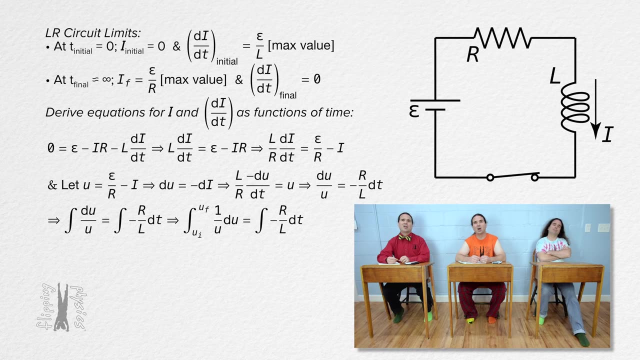 side where we are taking the integral with respect to the variable. u are just u initial and u final, Billy, what are the limits on the integral on the right-hand side of the equation? I'm not sure It's an integral with respect to time. 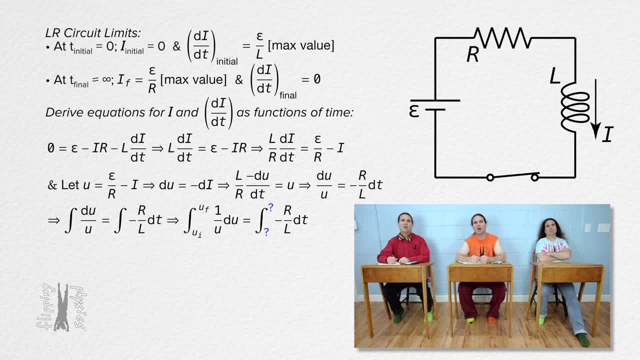 so I'm asking what the initial and final values for time in this integral should be. Okay, Time initial is when the switch closes, which is time equals zero. so the initial condition for time is zero. The final condition for time, well. 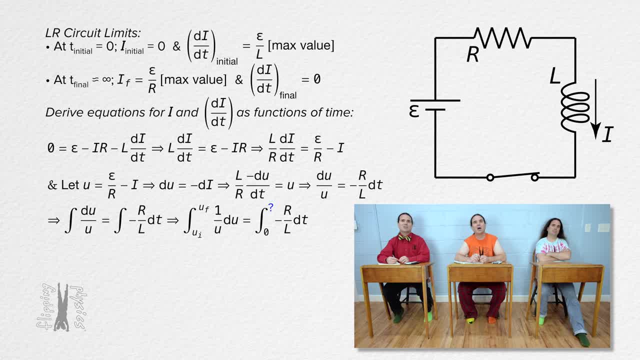 after a long time, the current is. Actually, we are not looking for what the current is after a long time. Remember, we are solving for equations for this L-R circuit as functions of time. Okay, I get it. Time varies from zero to time. t, The final value. 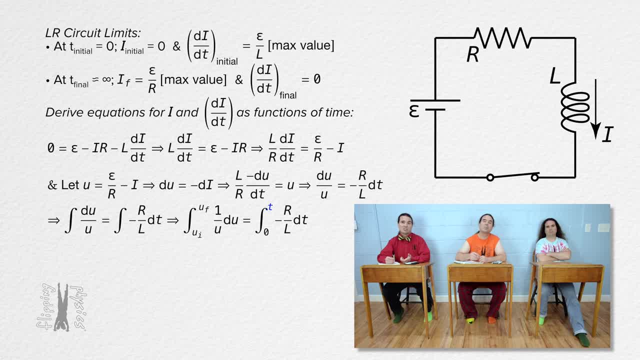 for time in these equations is the variable t, because we are solving for equations as function of time. So that makes sense. Thanks for your help, Mr P. You're welcome, Billy. Now let's take some integrals, starting on the left-hand side. 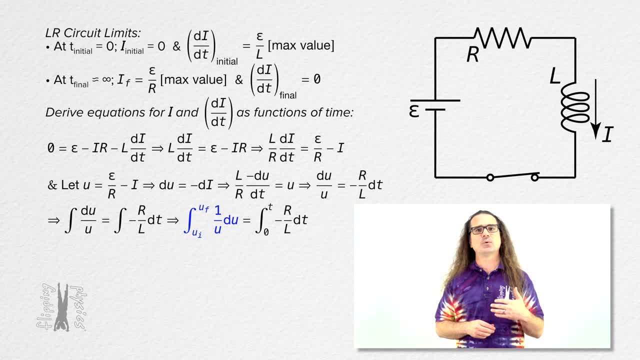 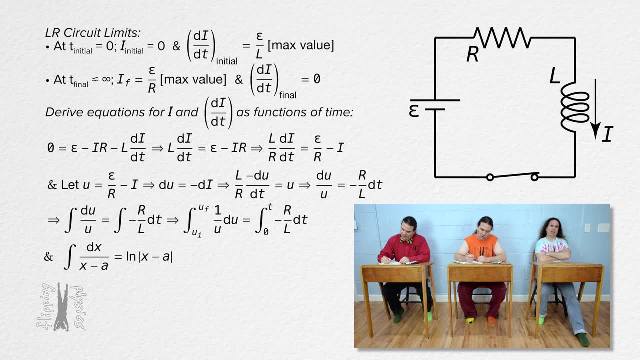 Bo, what is the integral of 1 over u with respect to u? equal to. We know the integral of the multiplicative inverse of x minus a constant. a with respect to x equals the natural log of the absolute value of x minus the constant. 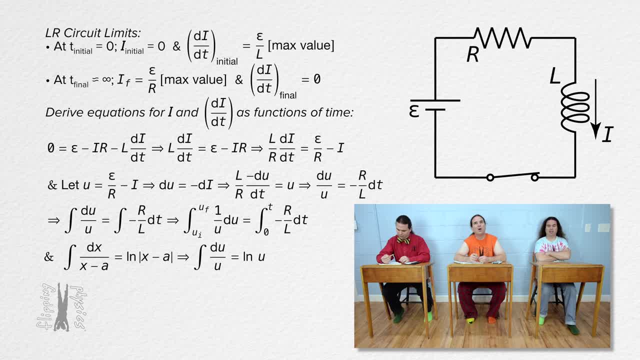 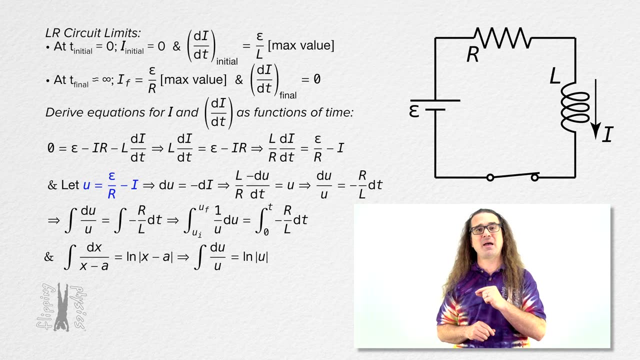 So the integral of the multiplicative inverse of u with respect to u equals the natural log of u. Wait, what happened to the absolute value? In this case? u equals emf divided by resistance minus current, and current varies from zero to emf divided by resistance. 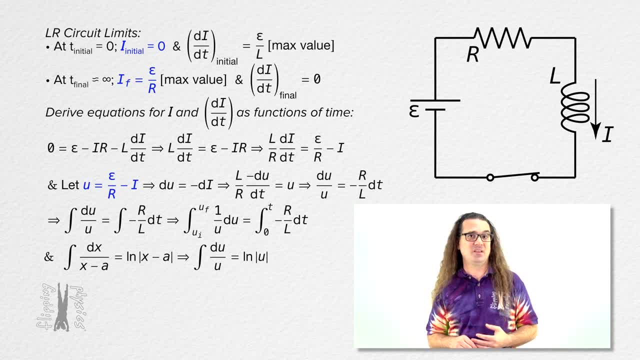 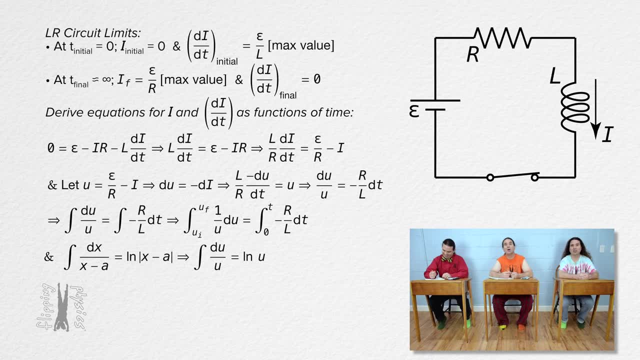 That means the variable u is never negative. Therefore we can remove the absolute value from the natural log of a constant a. So the integral of the multiplicative inverse of u equals the natural log of u. Then the left-hand side of the equation is the natural log of u. 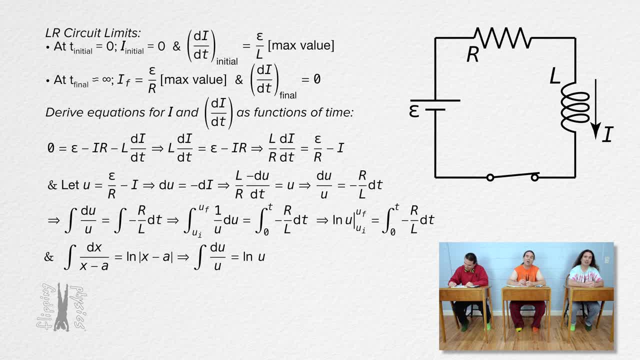 from u initial to u final And the right-hand side of the equation. well, resistance and inductance are constants and can be taken out from the integral, and the integral of 1 with respect to time is just time, Billy. please work on it from here. 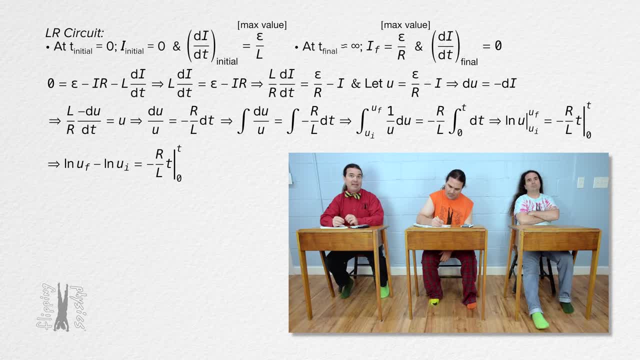 Absolutely. Let's substitute in initial and final conditions on the left-hand side, the natural log of u final minus the natural log of u initial initial equals the natural log of u final divided by u initial. Substituting in limits on the right hand side gives us negative resistance divided by inductance times time. This is: 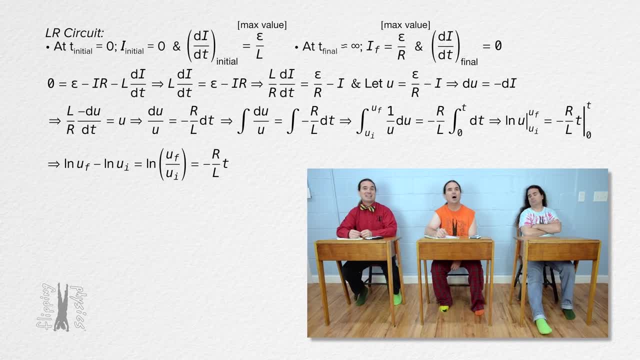 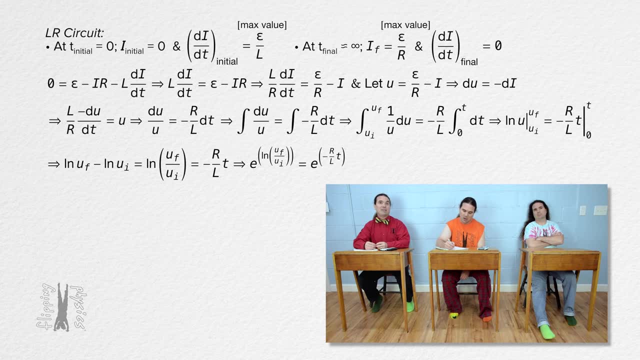 just like deriving RC circuits and drag force equations, because now we take e to the power of both sides On the left hand side, e to the power natural log of u final divided by u initial is just u final divided by u initial. We can multiply both sides by u initial from. 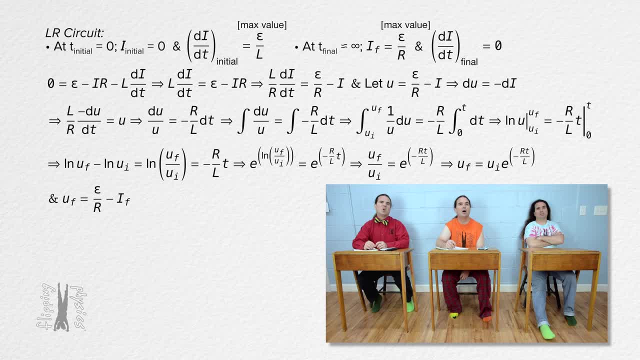 here u final equals emf over resistance minus current final and u initial equals emf over resistance minus current initial. However, current initial equals zero, So u initial actually equals just emf over resistance. Cool Thanks, Bo Yeah. 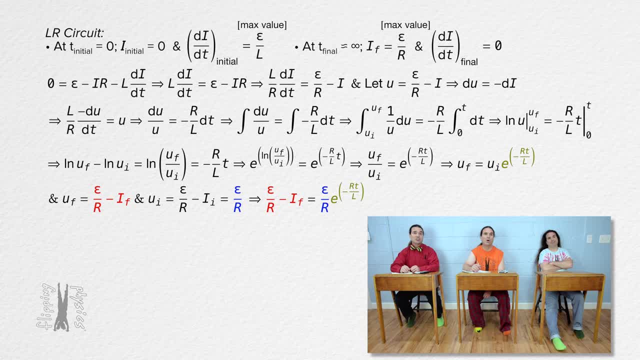 We can substitute those equations in for u final and u initial. Move emf divided by resistance to the right hand side, Multiply through by negative 1 and factor out emf divided by resistance and we get that the current as a function of time in this LR circuit equals emf divided. 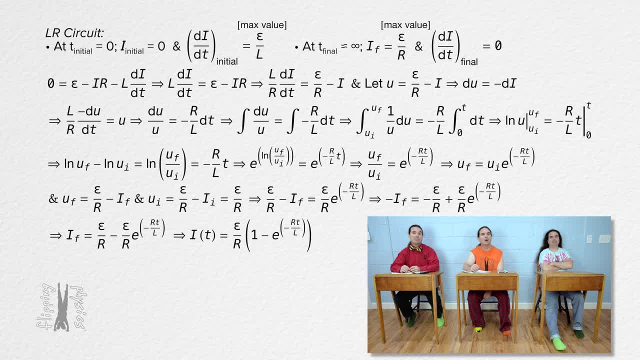 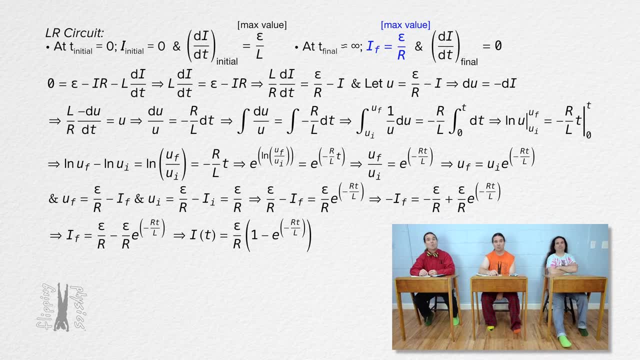 by resistance times. the quantity 1 minus e to the power negative resistance times, time divided by inductance And emf over resistance is the maximum current in the circuit. So you could substitute the current maximum into the equation if you wanted to. 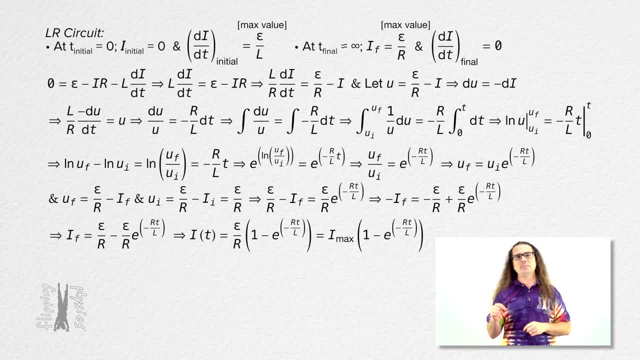 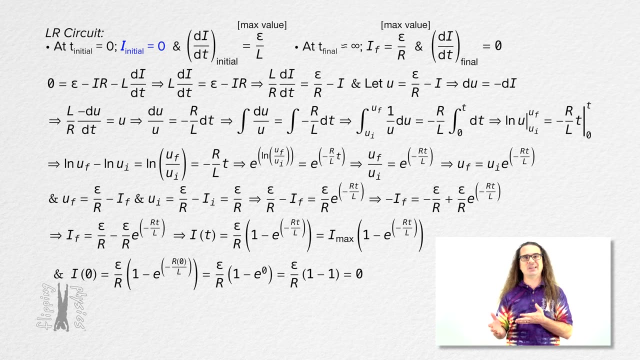 Absolutely Well done. Notice: this fits our limits for current because when we substitute zero in for time in our current, as a function of time equation, we get e to the power, zero, which equals 1.. And 1 minus 1 equals zero. and we already showed that the current in 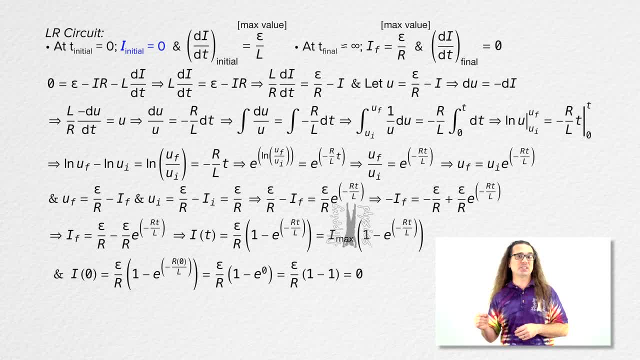 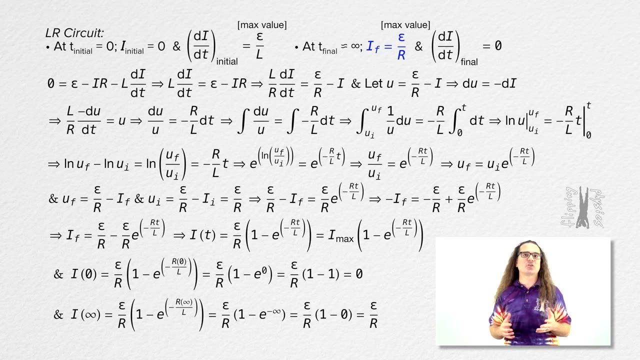 the LR circuit starts with a value of zero And when we substitute infinity into the same equation, we get e to the negative infinity, Which equals zero, Which gives us emf divided by resistance for the final current in this LR circuit after a long time, which again matches what we determined earlier for that. 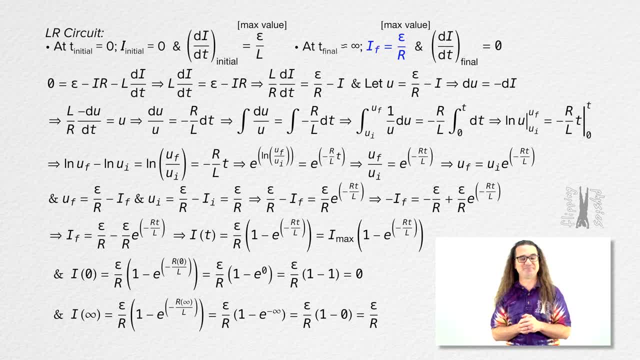 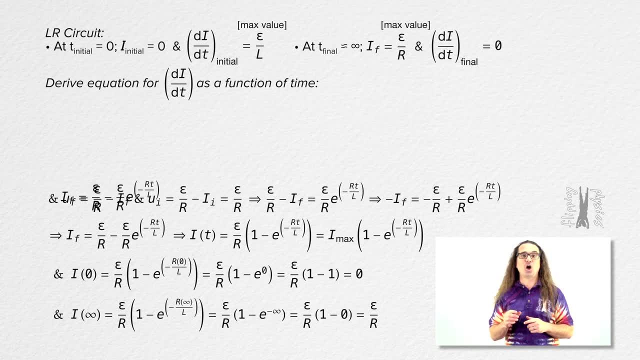 final steady state current in the circuit Nice, Yep, And we can also determine the time rate of change of current as a function of time. All we need to do is take the derivative of the current equation. we already derived Bo. what do we get when we take that derivative? 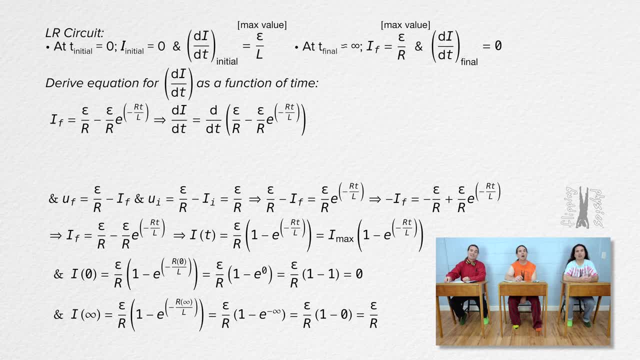 Sure, The derivative with respect to time of emf over resistance minus emf over resistance times e to the power negative resistance times time over inductance. Well, emf and resistance are both constants, so the derivative of emf over resistance with respect to time is zero. 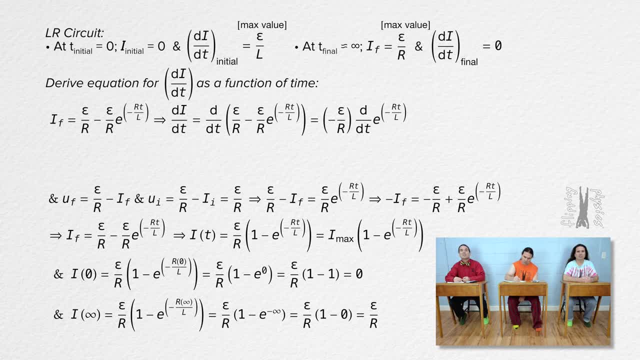 And negative emf over resistance can be taken out of the derivative. The derivative with respect to time of e to the power, negative resistance times time over inductance equals …. Well, we know. the derivative of e to the power, a times x with respect to x equals: 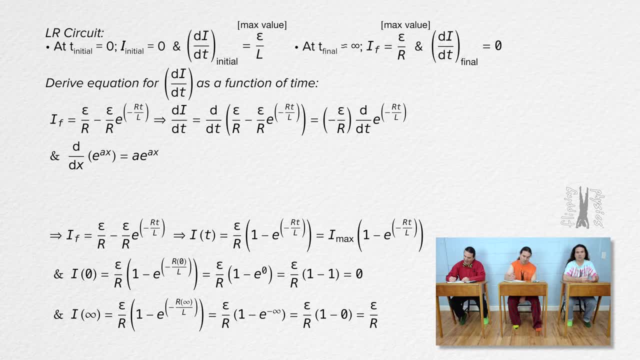 a times e to the power a times x. So the derivative with respect to time of e to the power negative resistance times time over inductance equals negative resistance over inductance times e to the power. negative resistance times time over inductance Resistance cancels. 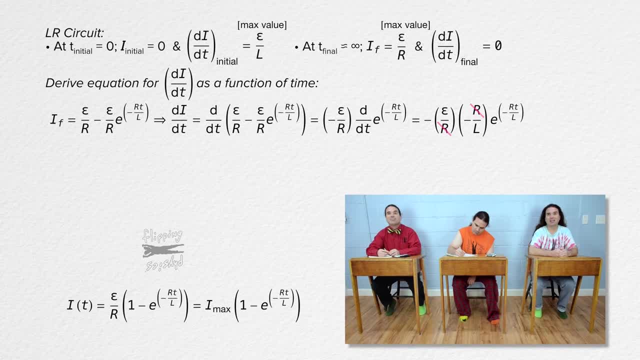 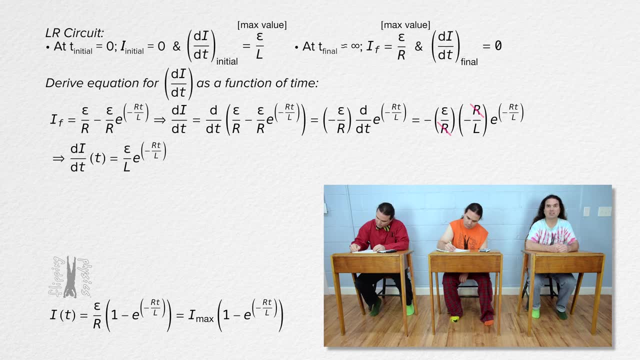 out …. … positive. And we get that. the time rate of change of current as a function of time equals emf over inductance times e to the power negative resistance times time over inductance. And we already showed that emf over inductance is the maximum value for the time rate of change. 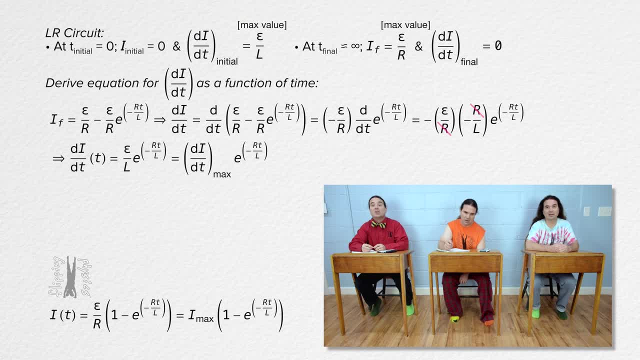 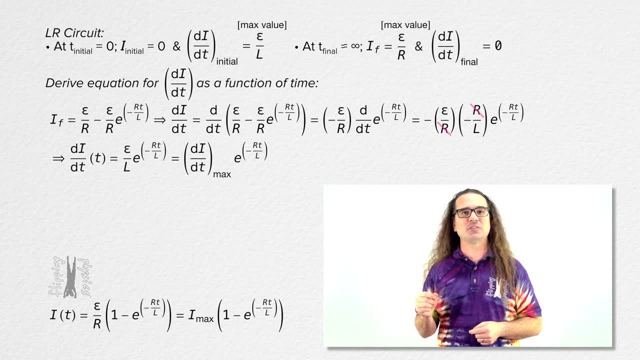 of current in this LR circuit, So we can substitute that into the equation. Excellent, Bo, Thank you. Yeah, again, notice that this fits our limits, because when we substitute zero in for time, we get e to the power, zero, which gives us the initial time rate of change of current. 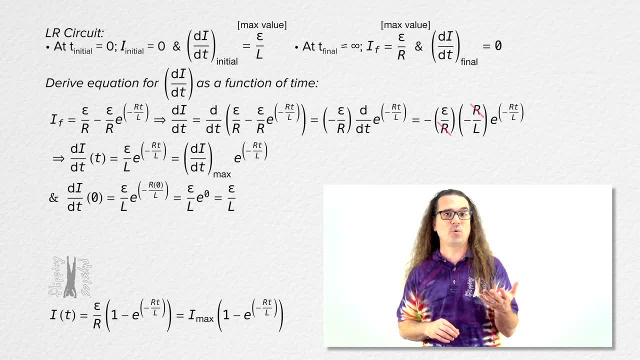 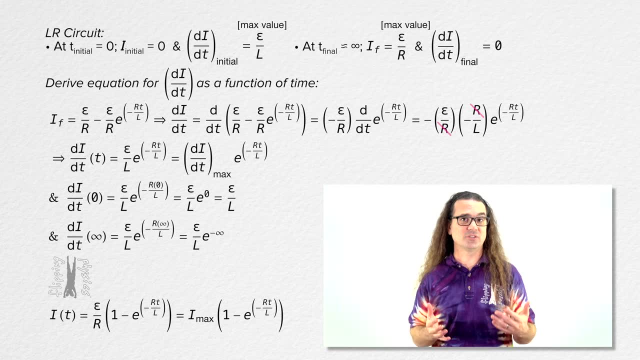 equals emf divided by inductance, which is what we derived earlier. And when we substitute infinity in for time, we get e to the power negative infinity, which is zero, which means we get zero for the time rate of change of current after a long time Again. 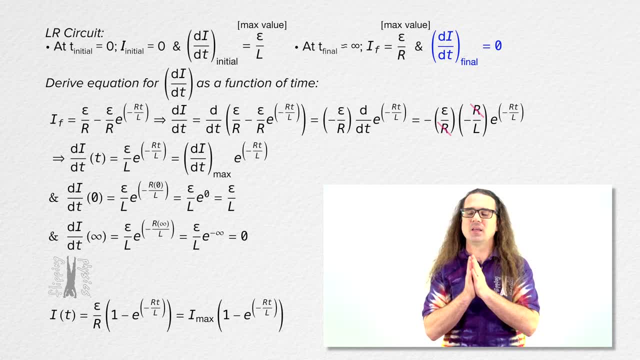 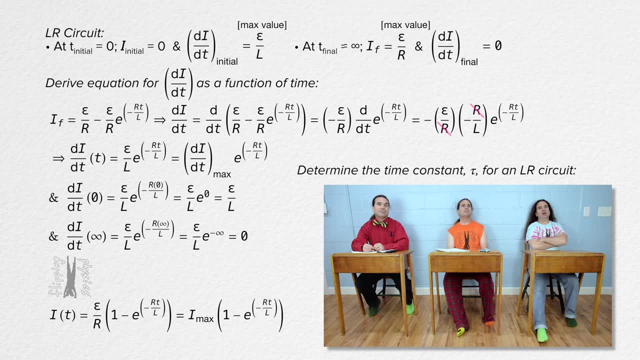 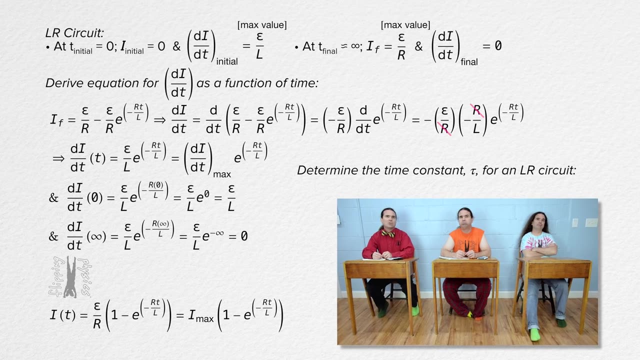 exactly what we derived earlier. Now, Bobby, please determine what the time constant for an L-R circuit equals. The time constant for an L-R circuit, uh, Remember, in these types of equations the time constant goes in the denominator of the expression which e is raised to. 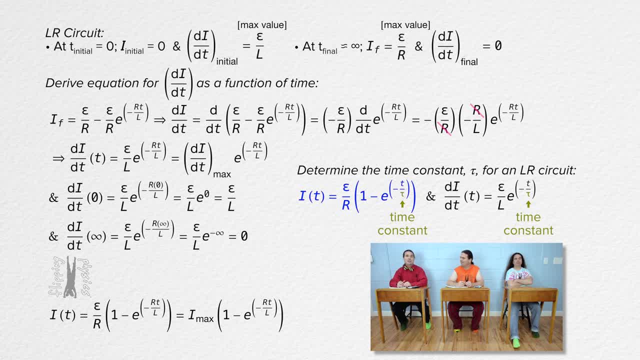 Uh, that means current as a function of time equals emf divided by resistance times, the quantity 1 minus e to the power negative time over time constant And the time rate of change of current as a function of time equals emf over inductance. 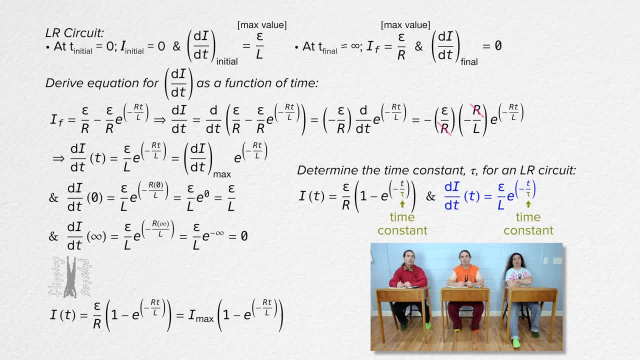 all times. e to the power negative. time over time constant. Okay, that means the time constant equals inductance over resistance. Yeah, for an L-R circuit we just showed that the time constant equals inductance over resistance. Right, But what is the time constant? 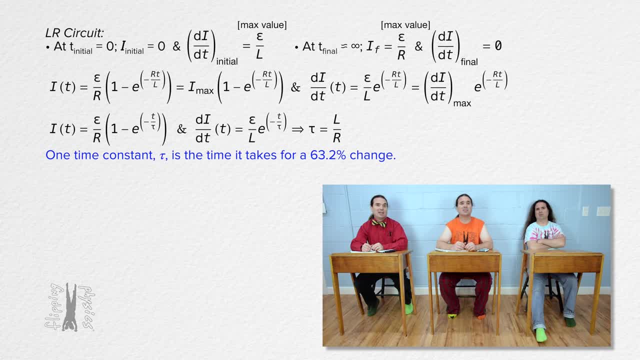 Oh, I remember that. Uh, Okay, One time constant is the time it takes for a 63.2% change. How do you remember that Mr P told us that one time constant representing the time for a 63.2% change in the variable. 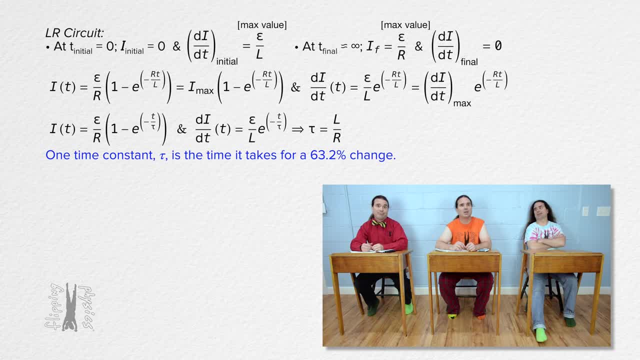 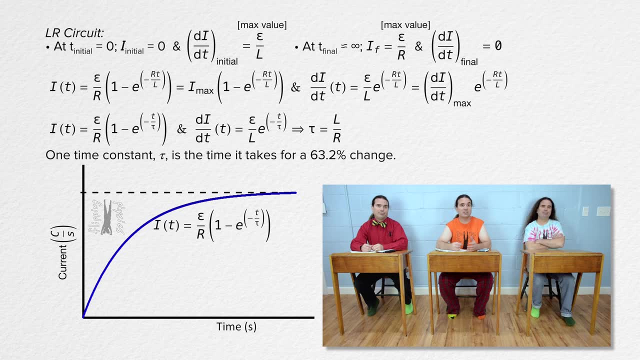 was an important number to remember, Right? Thanks, Um, if you look at the time constant in terms of graphs for current as a function of time, the current starts out at zero. increases, according to our equation and asymptotes, at a value of emf over resistance, the value of the final steady-state current in this. 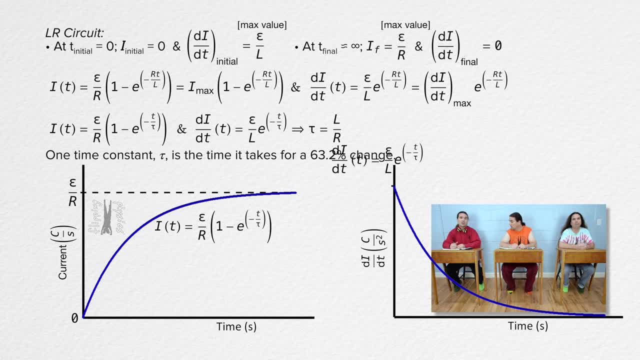 L-R circuit And the time rate of change of current starts out at a value of emf divided by inductance decreases, according to our equation, and asymptotes at zero the final value for the time rate of change of current in this L-R circuit. 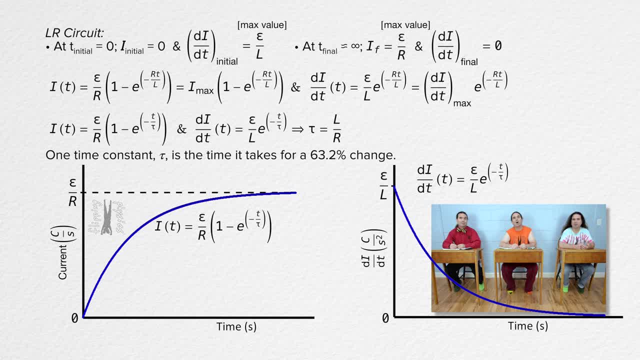 Okay, but it sounded like you were going to talk about the time constant and those graphs. Oh yeah, Uh. after one time constant of time has gone up, the time constant is going to go down. After one time constant of time has gone by, the current in this L-R circuit equals emf. 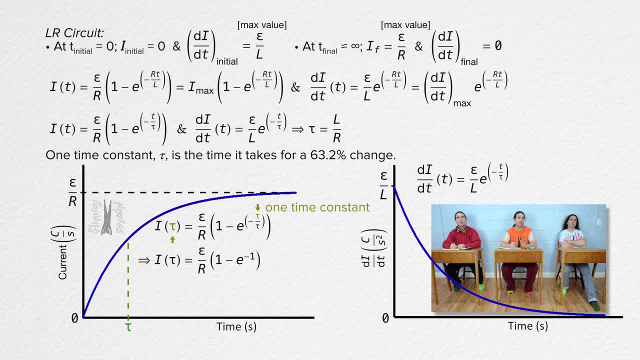 over resistance times. the quantity 1 minus e to the power negative 1, and e to the power negative 1 equals 0.368, and 1 minus 0.368 equals 0.632.. That means the current, after one time constant of time has gone by, equals 0.632 times emf. 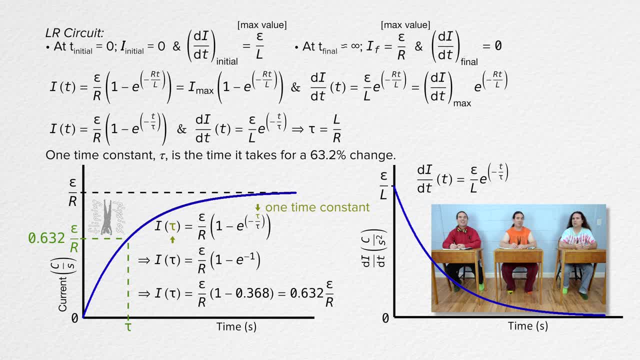 over resistance, or 63.2% of the final maximum current in the circuit, And after one time constant of time has gone by, the current in this L-R circuit equals 0.632.. After one time constant of time has gone by, the time rate of change of current in. 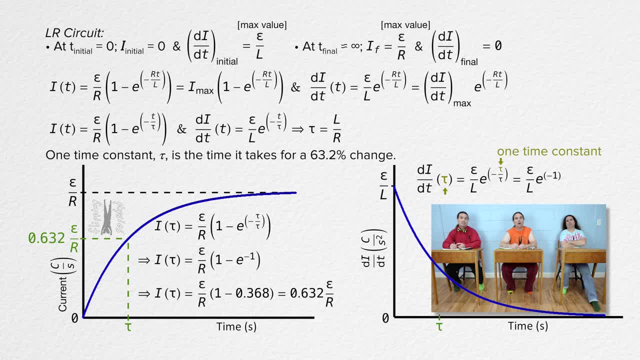 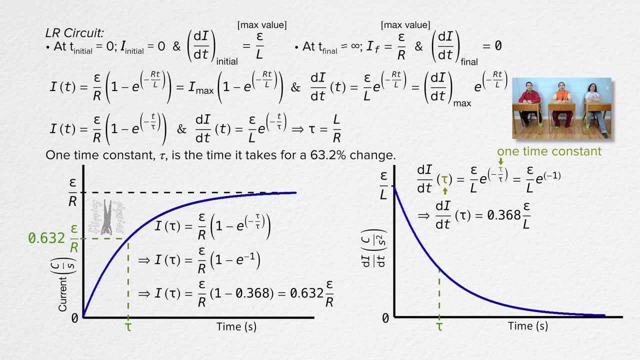 this L-R circuit equals emf divided by inductance times e to the power negative 1.. That means that after one time constant of time has gone by, the time rate of change of current in this circuit equals 0.368 times emf divided by inductance. 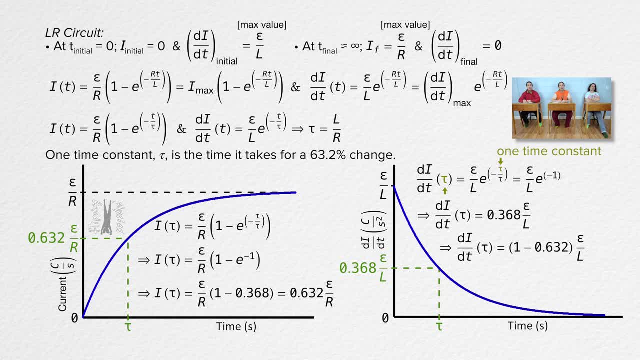 In other words, because 1 minus 0.632 equals 0.368,, the time rate of change of current in this L-R circuit has decreased by 63.2% from its initial maximum value. Okay, sure I get all that. 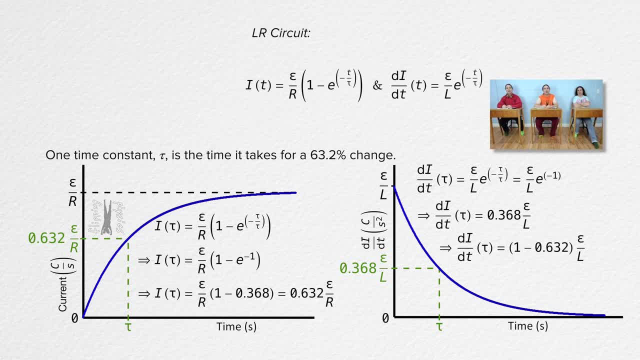 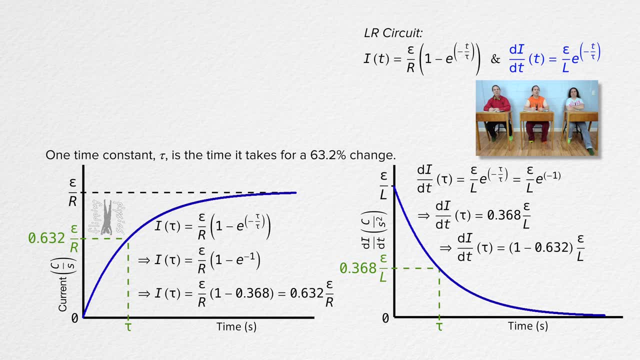 But what does it even mean that we have an equation for the derivative of current as a function of time, As a function of time? What, Yeah? what does an equation for the time rate of change of current as a function of time mean? 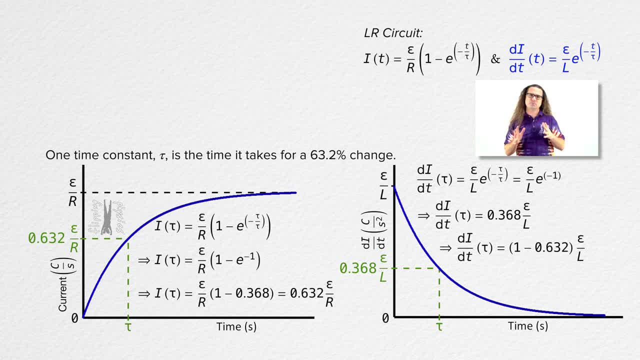 Sure, that is a fair question. So you can conclude that the derivative of current as a function of time is equal to the time rate of change of current as a function of time. What? Well, let's consider the derivative of current with respect to time to be the electrical 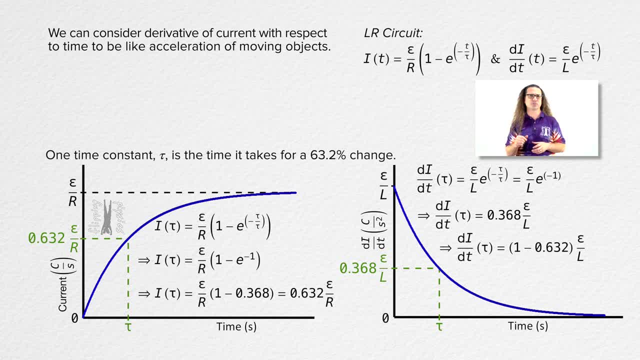 equivalent of acceleration for objects in motion. Okay, What? Okay, So current is in amps and amps are coulombs per second and velocity is in meters per second. So current in a circuit is like velocity for a moving object. 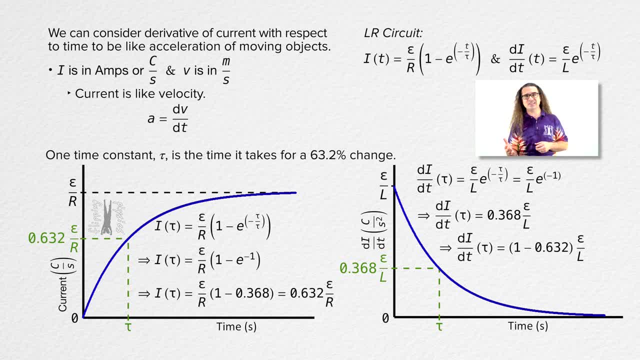 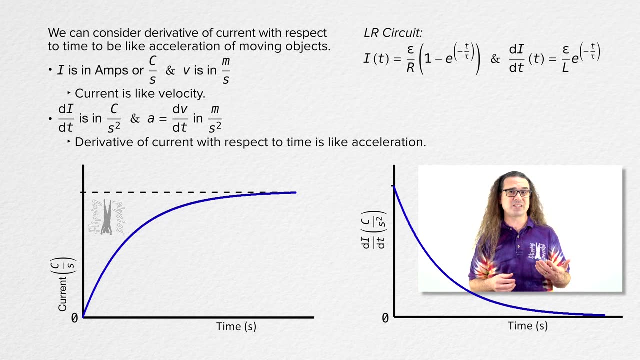 Okay, And the derivative of velocity with respect to time is acceleration. Acceleration has units of meters per second squared. The derivative of current with respect to time has units of coulombs per second squared. So the derivative of current with respect to time for a circuit is like acceleration. 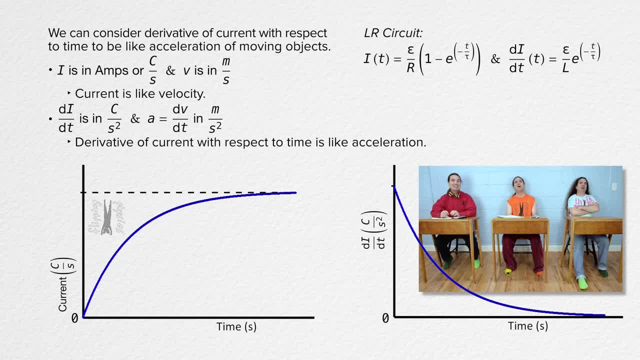 for a moving object. Okay, Okay. So, at the very beginning, the time rate of change of current is at its maximum value because the current is experiencing its greatest change with respect to time. The slope of current with respect to time has its greatest magnitude. 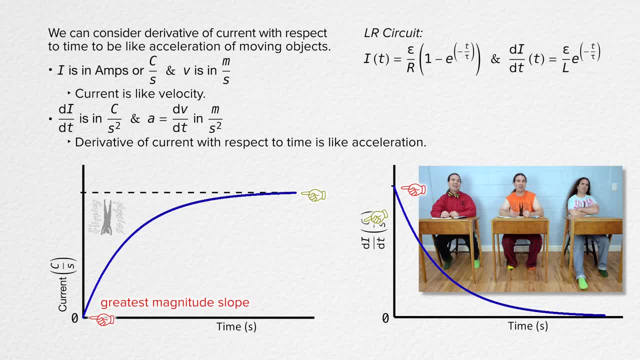 And at the very end, the current is not changing. Okay, The current is not changing. So the time rate of change of current as a function of time is zero, The slope of current as a function of time is zero, And these graphs are exactly the same as the graphs for velocity and acceleration as a 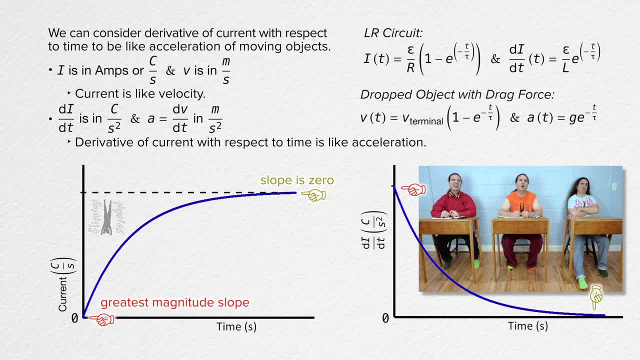 function of time for a dropped object which experiences a drag force. Whoa, OMG, You are absolutely right. The shape of the velocity curve is exactly the same as the current curve And the shape of the acceleration curve is exactly the same as the time rate of change. 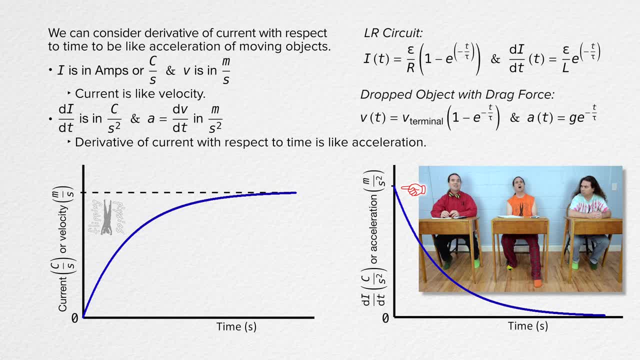 of current curve. So at the very beginning, the acceleration of the object in motion is at its maximum value because its velocity is experiencing its greatest change with respect to time, The slope of velocity with respect to time has its greatest value, And at the very end, the velocity of the object in motion is not changing. 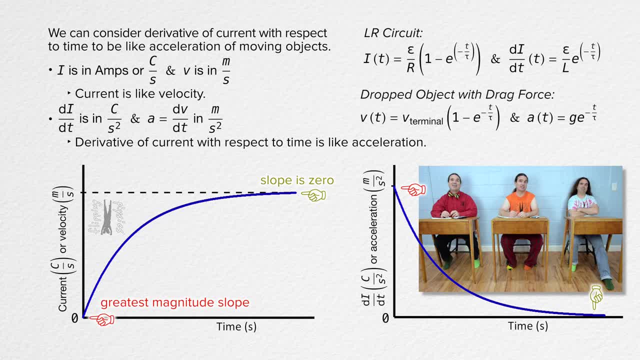 So the acceleration of the object is zero, The slope of the velocity with respect to time is zero. I get it, Mr P. That is what you meant when you said that we can consider the derivative of current with respect to time to be the alone. 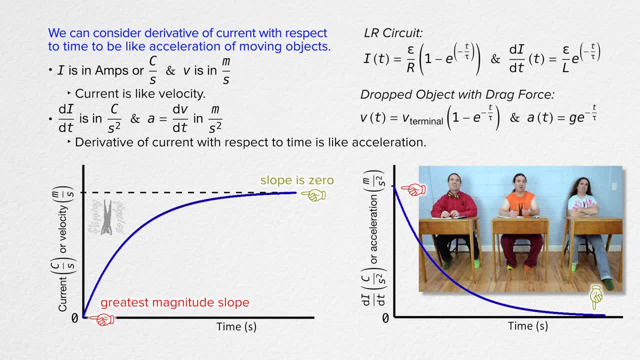 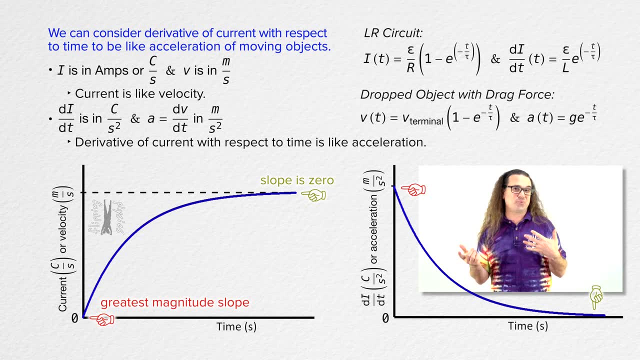 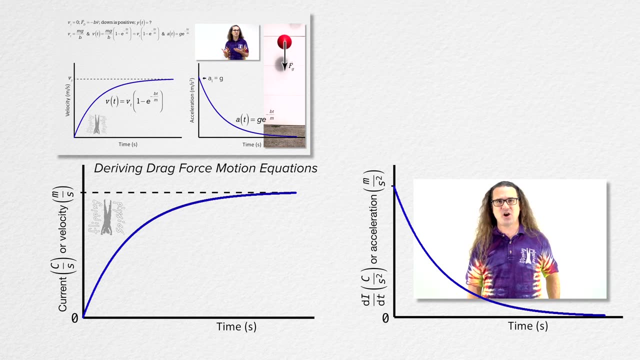 That is the electrical circuit equivalent of acceleration for objects in motion. That is cool, Trust me. Yeah, I know it's cool. And for the record, I just recycled the same graphs from my lesson Deriving Motion Equations with Drag Force and my lessons about RC circuits, because they are all the same graphs. 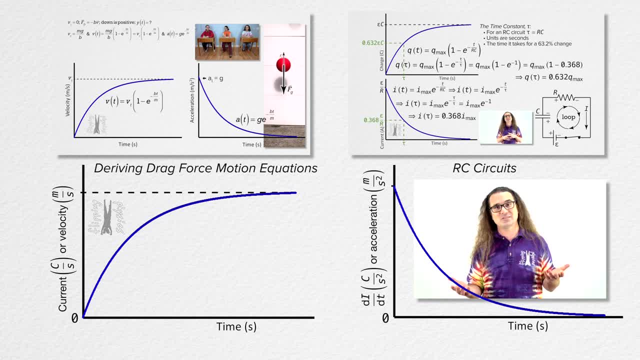 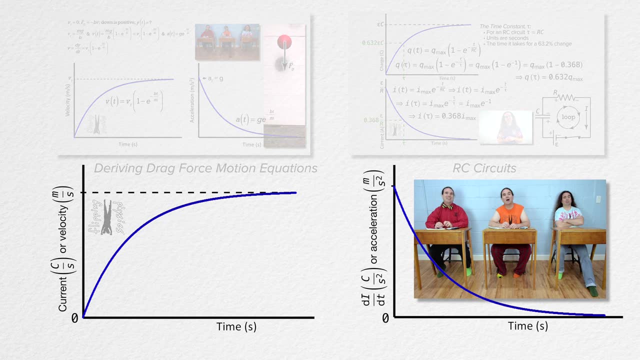 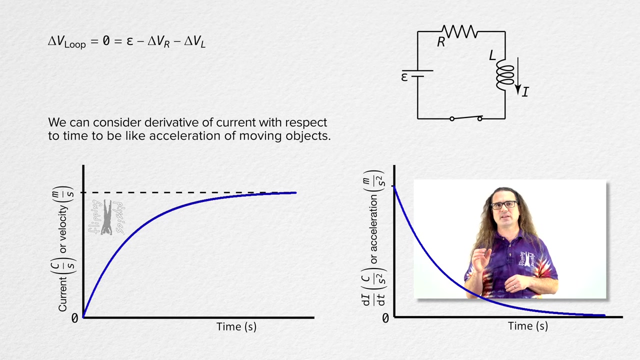 I just changed the labels on the vertical axes and the limits. Otherwise same graphs. Strange man. You know what we've gone this far? let's take the analogy just a bit further. Absolutely Sure. Looking at the L-R circuit, the equation we started with was zero equals emf minus electric. 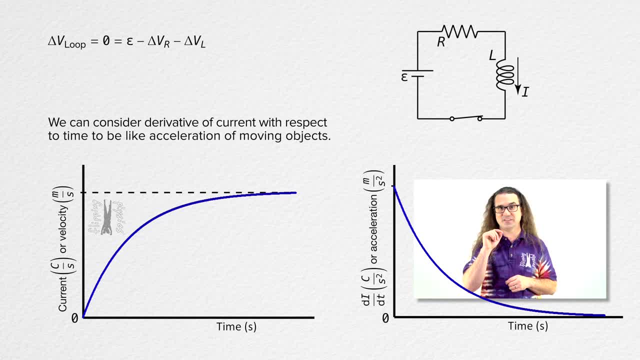 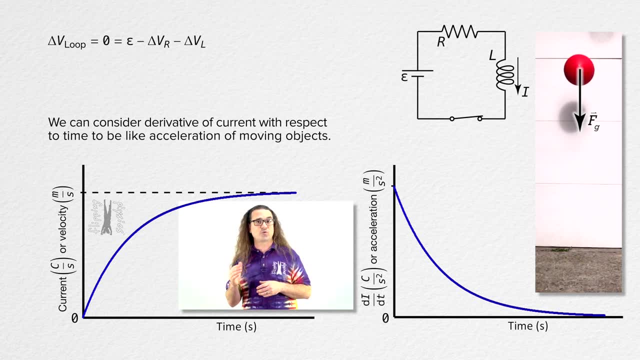 potential difference across the resistor minus electric potential difference across the inductor. Looking at an object released from rest and including air resistance, as the object falls, the force of gravity is down and the force of drag is up. In other words, the net force in the y-direction on the object equals taking the down direction. 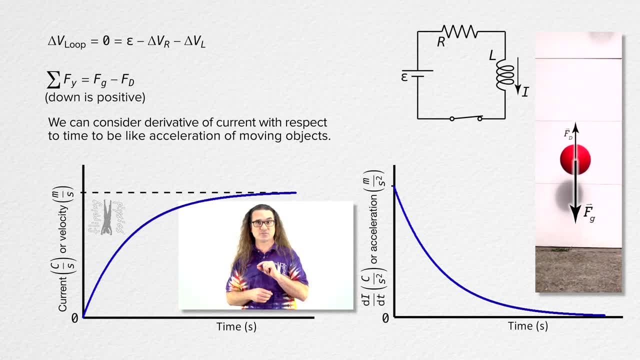 to be positive. force of gravity minus the force of drag And the net force in the y-direction also equals mass times acceleration in the y-direction And we can rearrange that equation to get zero equals the force of gravity minus the drag force minus mass times acceleration in the y-direction. 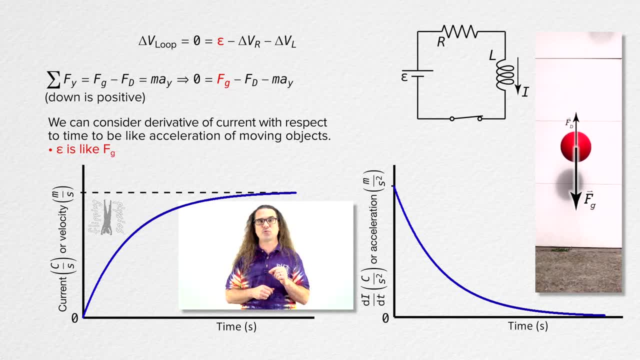 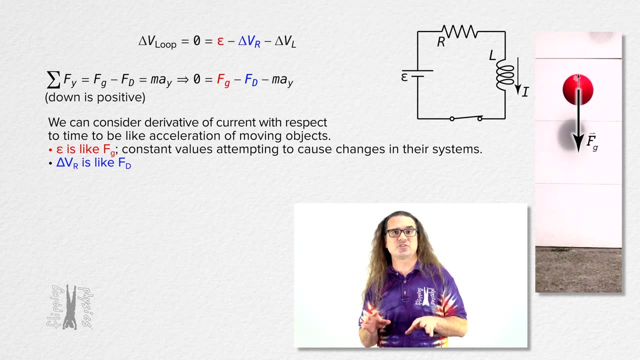 So the emf is analogous to the force of gravity. Both are positive, Both are constant values which are attempting to cause changes in the respective systems. Emf is attempting to change current, Force of gravity is attempting to change velocity. The electric potential difference across the resistor is analogous to the drag force. 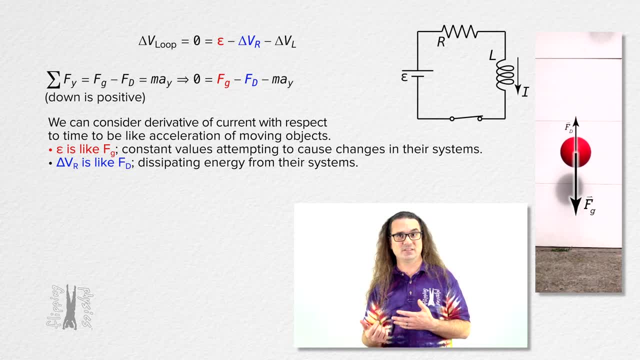 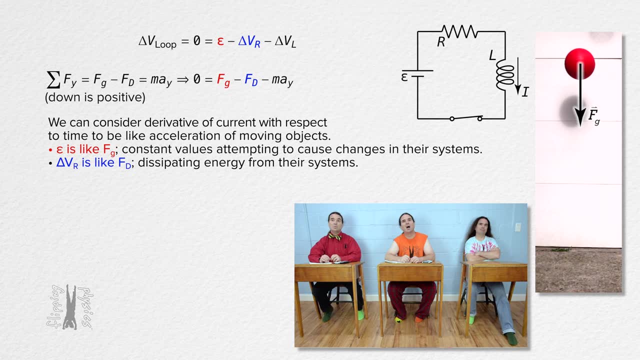 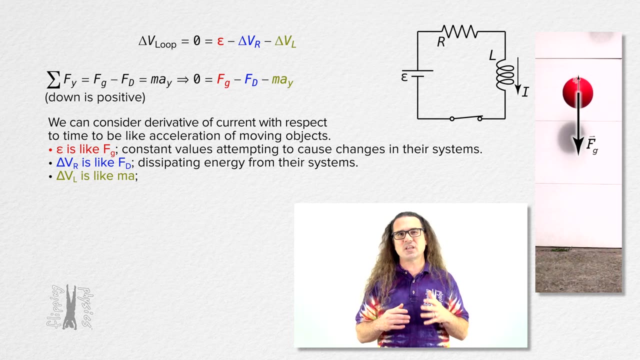 Both are dissipating energy from their respective systems. The resistor is converting electric potential energy to heat and the drag force is converting gravitational potential energy to heat. The electric potential difference across the inductor is denoted by solid energy゛n. inductor is analogous to mass times acceleration When we substitute inductance times the derivative. 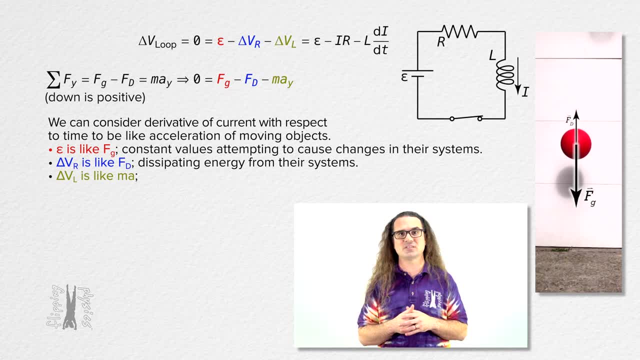 of current with respect to time in for the electric potential difference across the inductor and the derivative of velocity with respect to time in for acceleration. you can see that inductance is analogous to mass. Inductance opposes changes in current. Mass opposes changes. 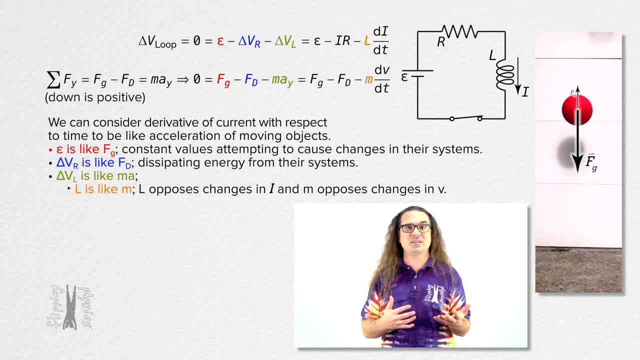 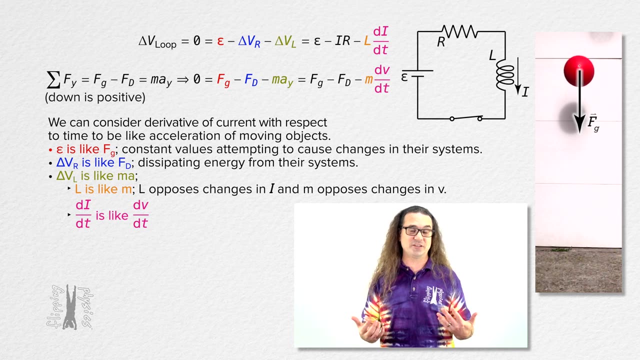 in velocity, because mass is a quantitative measure of inertia, and inertia is the tendency of an object to resist acceleration, And the derivative of current with respect to time is analogous to the derivative of velocity with respect to time or acceleration, which is what I meant when I said we can consider the derivative of current with respect to time to be the electrical